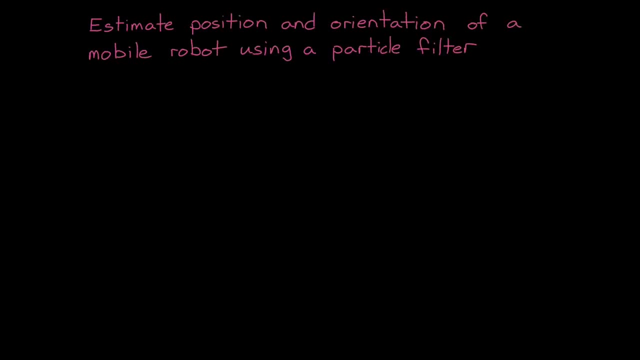 In the first video, we talked about what autonomous navigation is and how it can be applied to different types of autonomous vehicles. In this video, we're going to look at one part of autonomous navigation and show how you can estimate the position and orientation of a mobile robot using 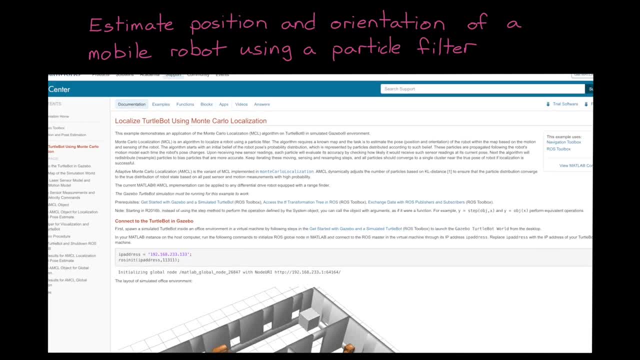 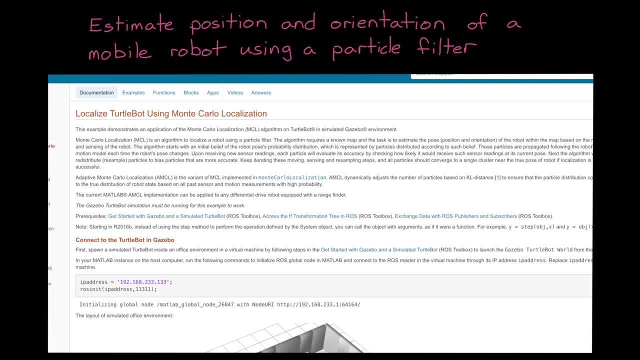 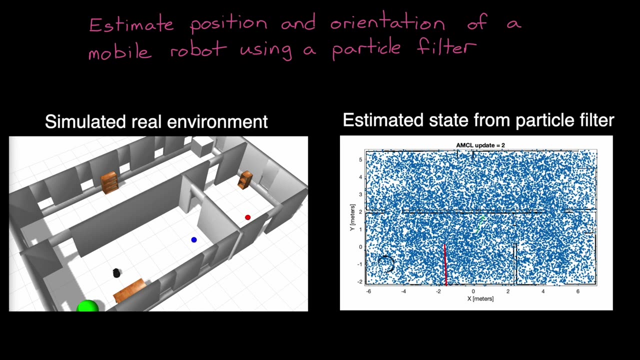 a particle filter. We're going to go through the same localization approach as demonstrated in the MATLAB example: localized turtle bot using Monte Carlo localization. This example simulates a turtle bot moving around in an office building taking measurements of the environment and estimating its location, And if you're not familiar with a particle filter, it may be. 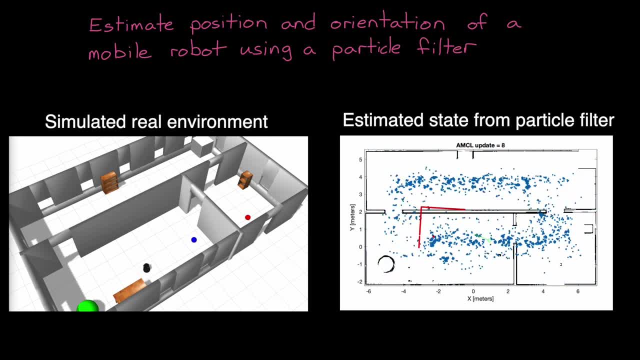 confusing as to why the solution has a bunch of blue dots appearing and jumping around each time step, and then somehow converging on the real location of the turtle bot. What is this filter doing, and how does this seemingly random set of dots help us determine the location of a robot? 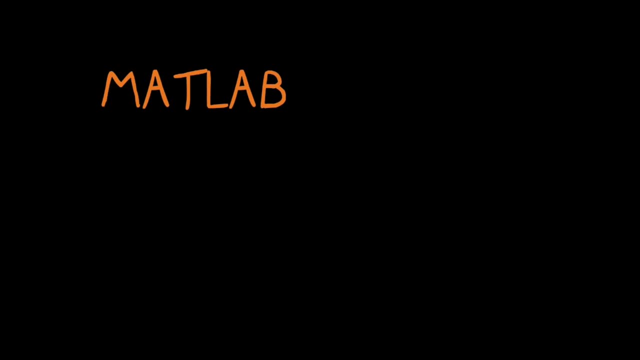 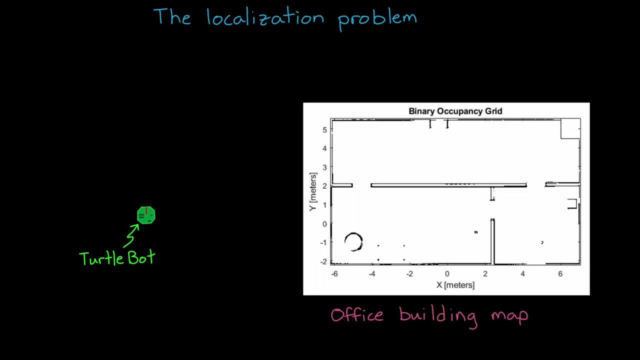 That's what we're going to cover, so I hope you stick around for it. I'm Brian, and welcome to a MATLAB Tech Talk. Let's set up the localization problem. We have a robot- the turtle bot- that's wandering around inside an office building. The robot is given a map of the building so it knows the general layout. 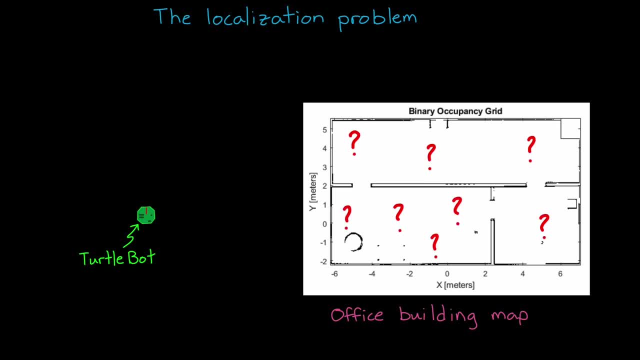 of the walls and the furniture, but it doesn't know initially where it is within the map. It could be anywhere. Therefore, the problem is that the robot needs to use its sensors and motion models to estimate its pose, That is, determine its position and orientation within the building. 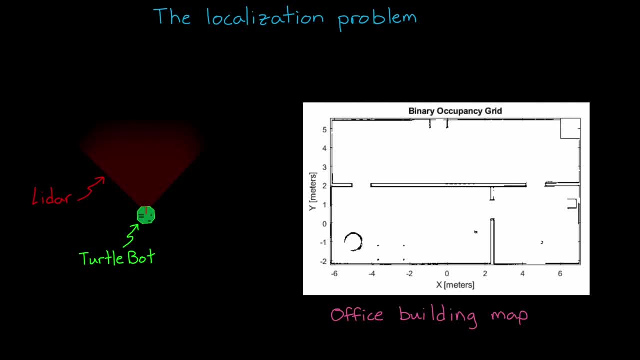 This robot has a lidar sensor that returns the distance to objects within the field of view. So if the sensor is looking at a corner and two doors, it might return a point cloud of dots that looks something like this, But measurements are actually noisy, so it really might look. 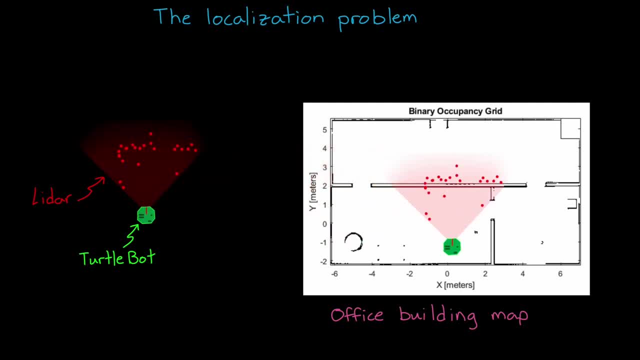 something like this. Now we can match this pattern to the map of the environment and determine where the robot is Now. in addition to a noisy measurement, the robot also has a way to dead reckon its position using odometry data. Dead reckoning is when a future position is calculated. 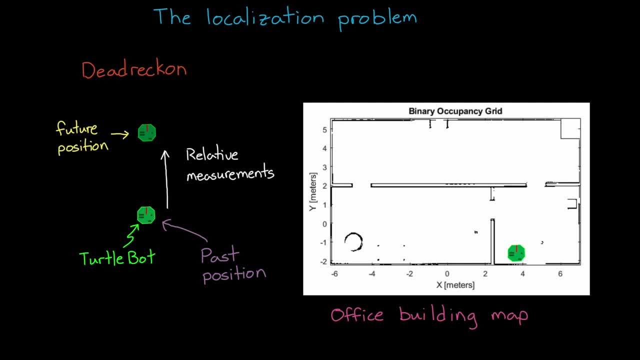 using a past position and relative measurements like velocity and angular rate. So if you know that the robot is facing north and moving at one meter per second, then after three seconds you can estimate that the position is three meters north of where it used to be And you can have some 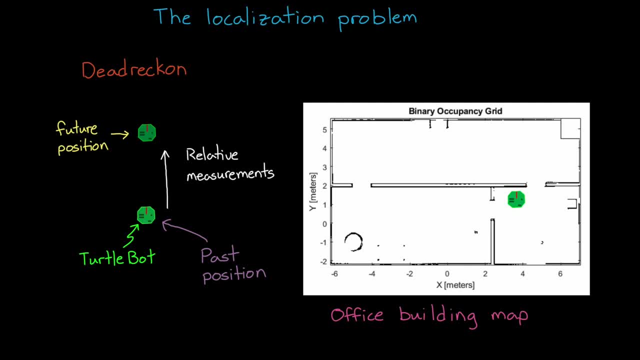 confidence that this is the case without having to check the environment again. Dead reckoning can be used over shorter time frames with a lot of success, but due to noise and the relative measurements, over time the error grows and needs to be corrected by measuring where it is relative. 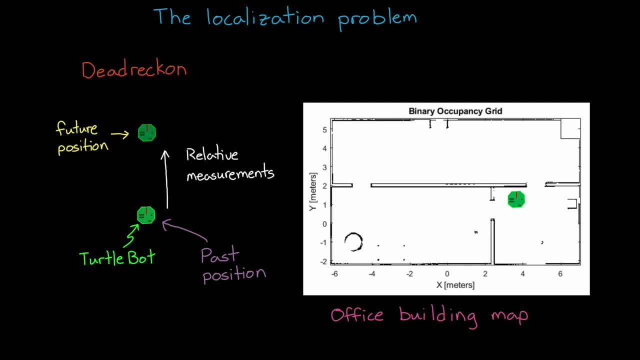 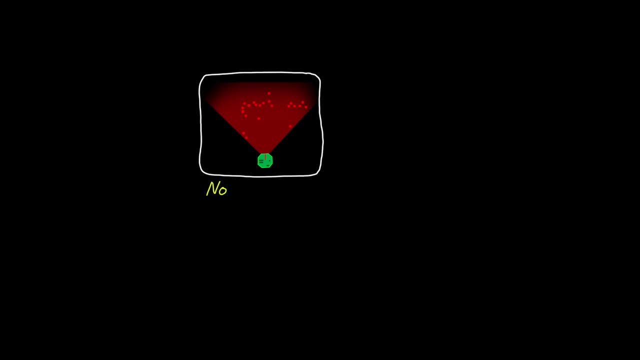 to the environment. For a more in-depth understanding of dead reckoning, check out the sensor fusion and tracking video number three, linked below, where we combine the absolute measurement from a GPS with the relative measurement from a robot, from an IMU, So we have two possible ways to determine location. We have a noisy 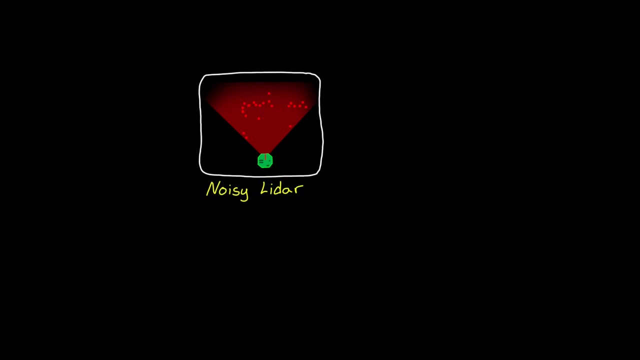 LiDAR sensor that senses features that we can compare to a map of the environment, and we have noisy odometry data that estimates how the robot is moving. Now, if you're familiar with the Kalman filter, you might recognize that blending a noisy measurement with a noisy process model is exactly what it's. 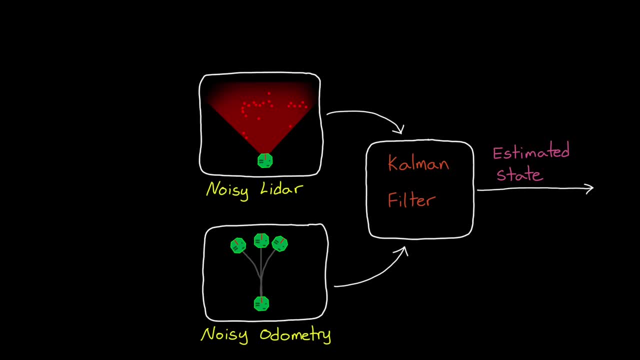 used for. And if you're not familiar with Kalman filters, you can get up to speed by watching the MATLAB Tech Talk series on them that I've linked to in the description below, but you really shouldn't need too much experience with them to understand the rest of the video. One drawback of a Kalman filter, that's 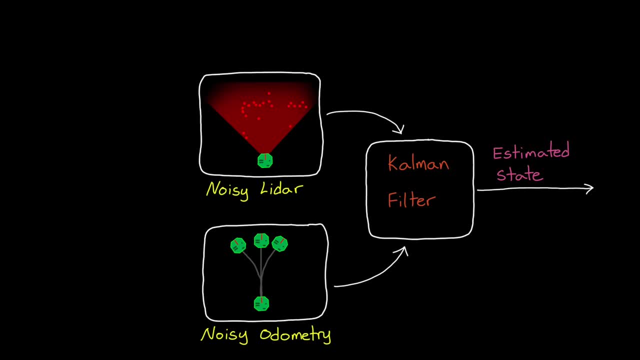 going to be important for us is that it expects probability distributions to be Gaussian. So for our problem, the random dead reckoning noise needs to be Gaussian and the LiDAR measurement noise needs to be Gaussian, which both might actually be, or at least close enough to be true. 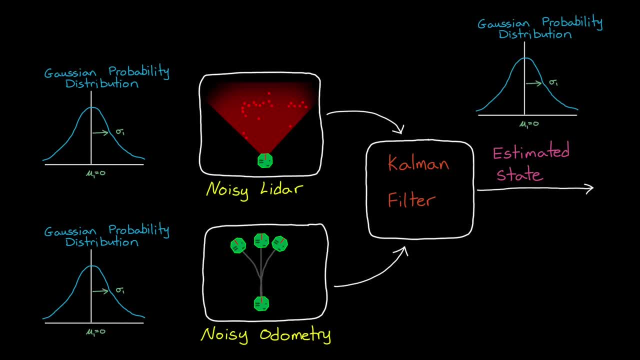 But, importantly, the probability distribution of the estimated state of the robot must also be Gaussian, which, we'll see in just a bit, is definitely not the case for our localization example. Therefore, we need an estimation filter that can handle non-Gaussian probability distributions. 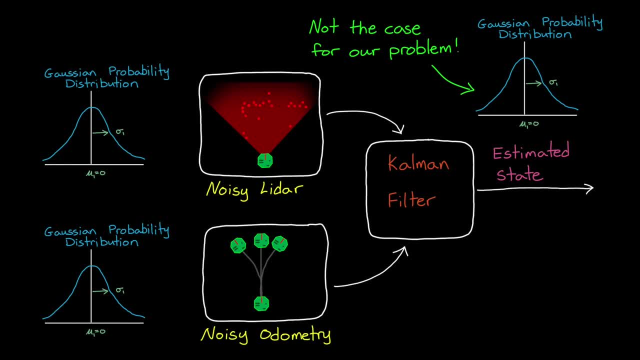 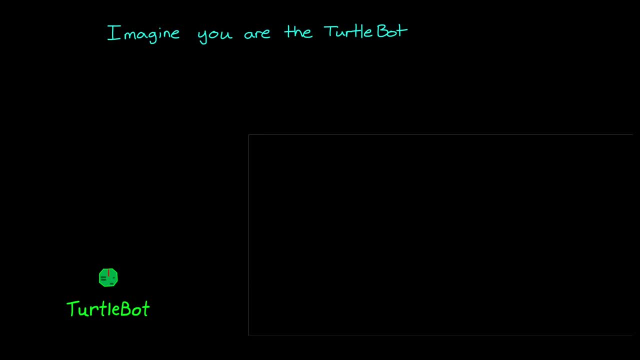 and that's where the particle filter comes in. To understand how the particle filter is going to solve our localization problem, we should try to imagine ourselves as the robot And figure out how we would use LiDAR to determine where we are on a very simple map. 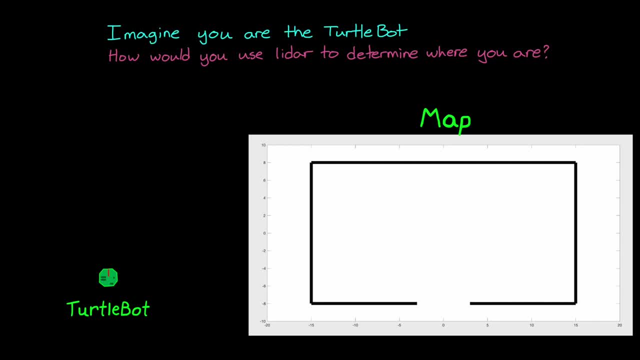 At the beginning, we have no clue where we are in the room. We might say that it is equally probable that we're anywhere on the map and facing any direction. At this point, we measure the scene with the LiDAR sensor and receive the result It. 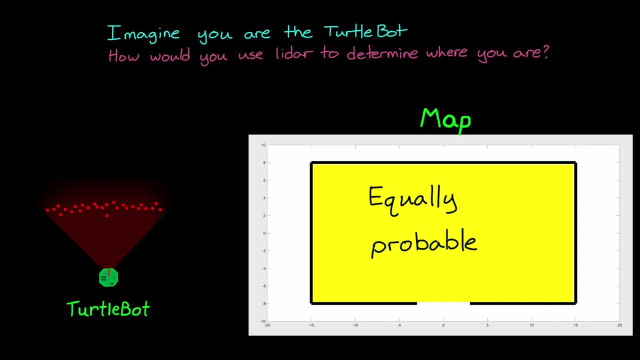 looks like we're looking at a wall, since all of the measurements are basically in a line and from that measurement we can tell about how far away we are from the wall. We can't tell from this alone our exact location, because there are many walls in this room and we might be facing any one of them or anywhere along. 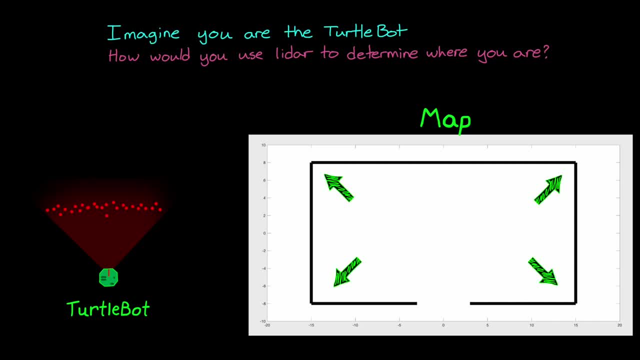 each of the walls, But we can tell that we're probably not looking at a corner or the door and we're probably not in the middle of the room, since the wall is so close. So this first measurement constrains us to maybe one of these. 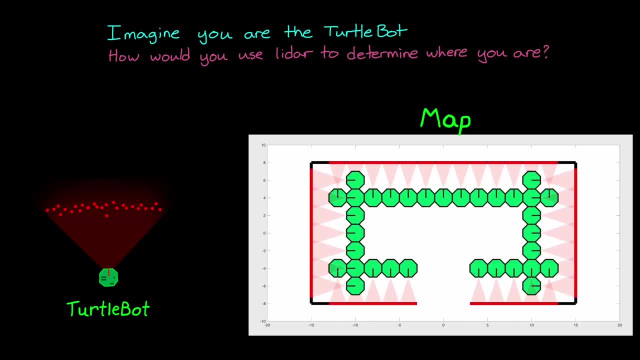 positions and orientations. However, since the sensor has some noise and error, we may claim that we could be a little closer or further away than the measurement states. So we can expand the possible locations accordingly and say that we have the most confidence that we're in one of these locations. Now we 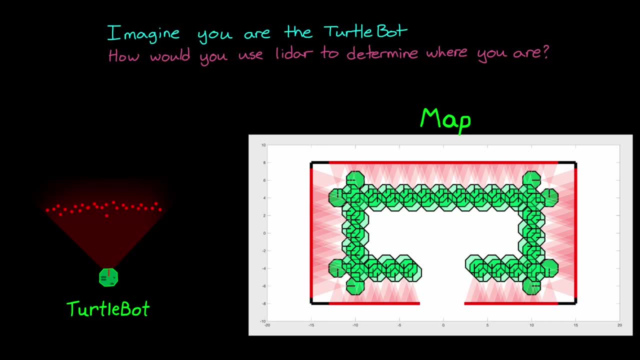 can't say for sure that we're not in the middle of the room, because it's possible that we're looking at a temporary flat obstacle that wasn't on the map. Likely, it's a lower probability that that's the case, but it's still possible. Therefore, 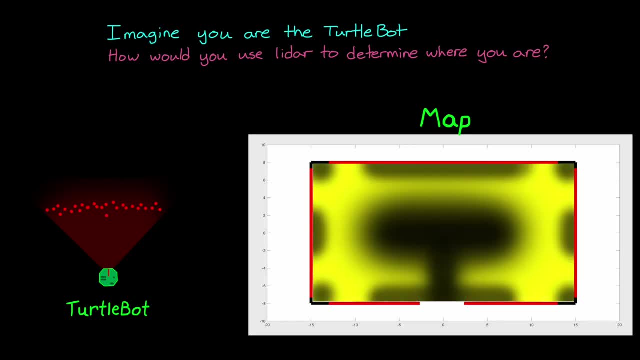 after this first measurement, we may say that the probability of the second measurement being the most likely is higher than the other. So we can see that our probability is lower than the other more often, And this is the same thing we saw before. The only difference is that the 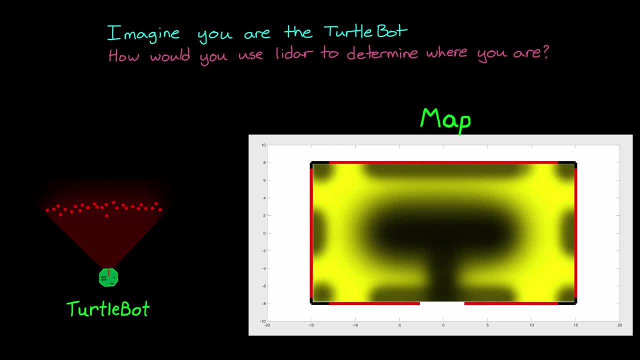 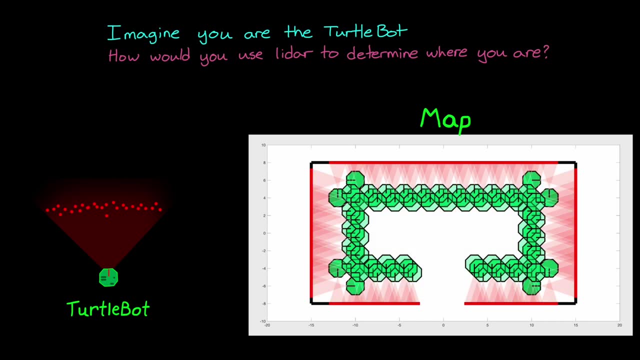 distribution of where we are looks something like this, with the brighter yellow locations meaning higher probability and the darker locations are lower probability. This is already a very non-Gaussian distribution. so you can see how easily we get ourselves into a non-Gaussian situation when we're dealing with localization like this. 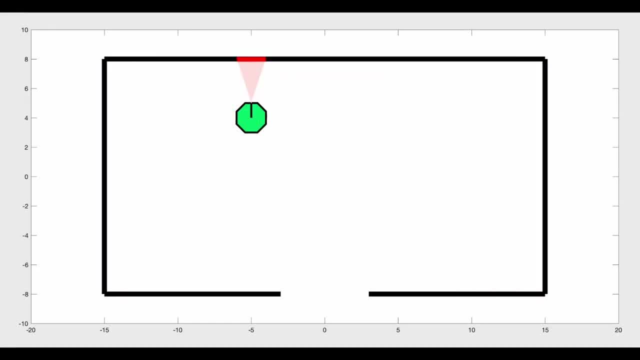 Okay, so intuitively, it makes sense that we can't be certain where we are from this single measurement. We're not going to take this simple measurement for granted, But let's say that this is actually where we are within the room. Again, we're still just looking at this flat, featureless wall. 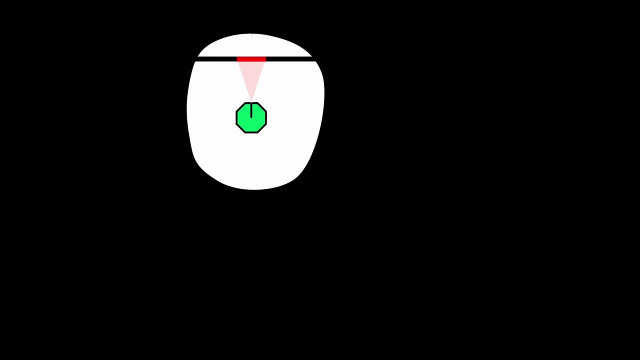 As a person, it makes sense that if we moved around to see different features, we could start to narrow in on exactly where we are by removing the locations that don't satisfy all of the measurements that we see along the way. So if we turn to the left and see a corner, 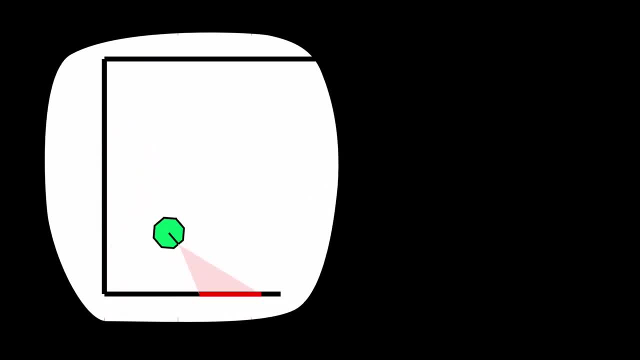 and then keep turning and see another corner and then we see the door. we would be able to use our memory to start to piece together where we are on the map, based on what we've seen and based on the estimate of how we moved through the environment. 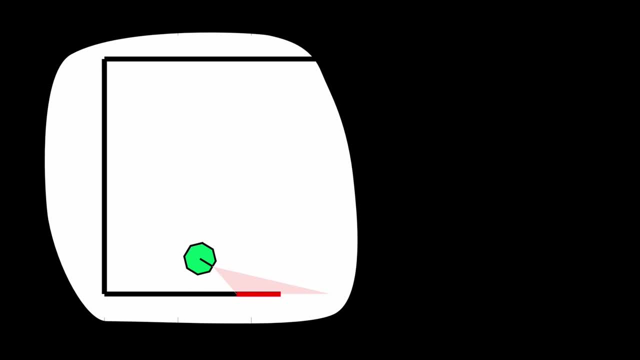 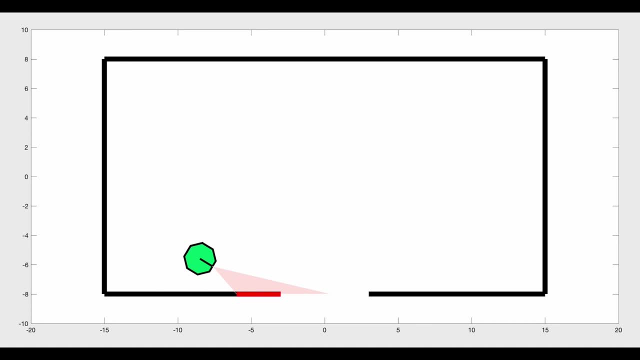 which is the direction we turned and about how far we walked, And there's only one place on this map where a motion like this will see exactly two corners and then end at a door. So this must have been the path that we took and this must be where we are now. 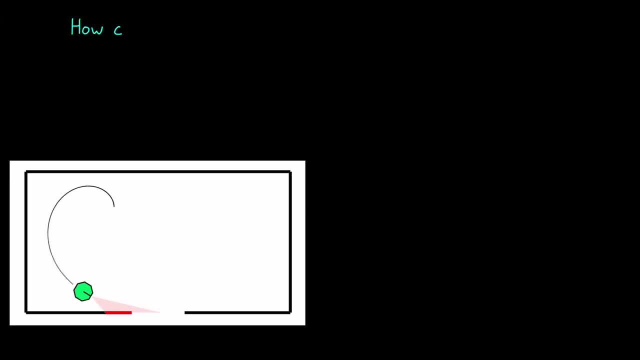 So this all makes intuitive sense, But how can we code this kind of understanding for our robot, How can it remember multiple successive measurements in a way that allows it to hone in on its exact location over time? Well, as you probably expect, since I already told you, 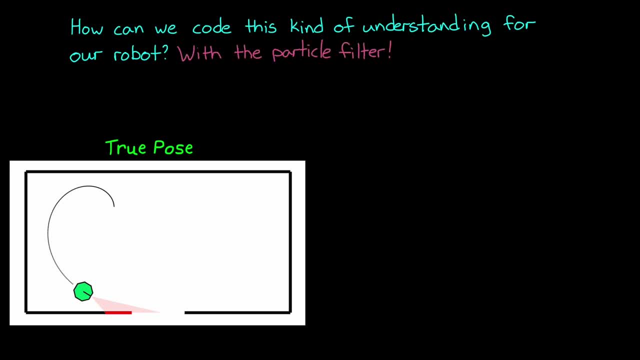 one popular way is with a particle filter. Now we're going to walk through a really basic understanding of how particle filters work. The goal of this section is to give you some intuition about the filter and not to go too in-depth into any of the mathematics. 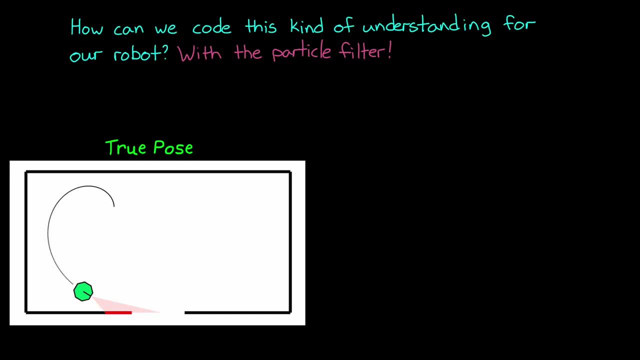 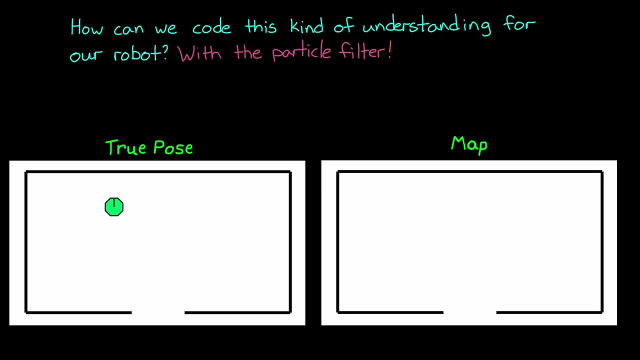 But first let's take a look at the particle filter. But if you want more details about the filter, I've left some great resources in the description. All right, let's get started. Remember, at the start the robot has a map of the room, but nothing else. 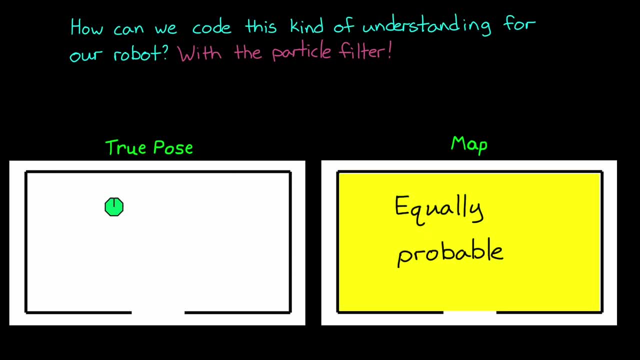 And so there is equal probability that the robot is anywhere on the map and facing any direction. So rather than try to capture this probability with some smoothly defined function, we can approximate the probability distribution by randomly generating a number of discrete poses. Here I'm uniformly randomizing the X and Y location. 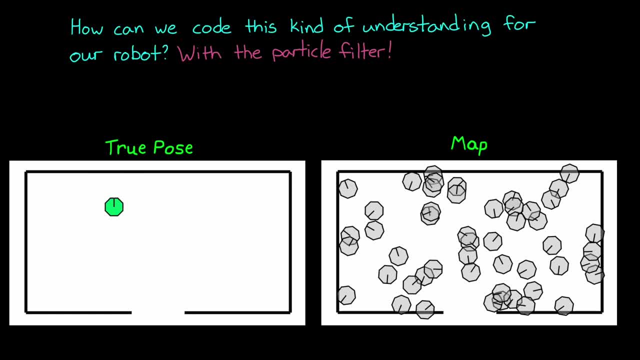 and uniformly randomizing the orientation using 50 different poses. This captures the uniform probability distribution across the entire map. Now each one of these poses or particles is saved in the filter as a possible estimate of the state, And the more particles, the closer they represent the true probability distribution. 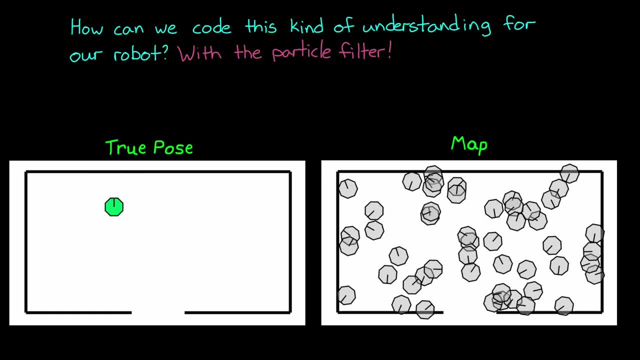 But the more time it takes to do all the calculations. so there's a trade-off between accuracy and speed. Now for this thought exercise, 50 particles will be enough, But you may need hundreds or thousands, depending on the size of the map. 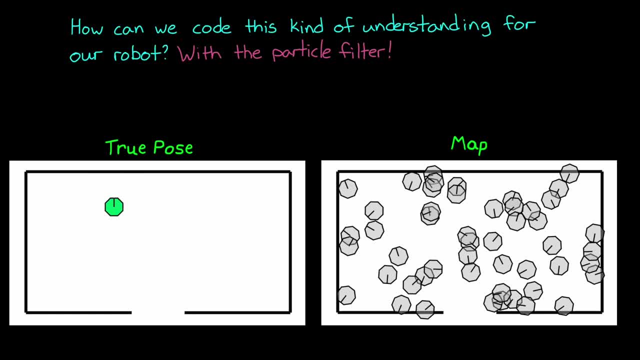 and the shape of the probability distribution that you're trying to represent. Now, a bunch of random guesses of system state doesn't seem like it helps us much, since so many of them clearly have to be wrong, But we can start to remove some of the wrong guesses. 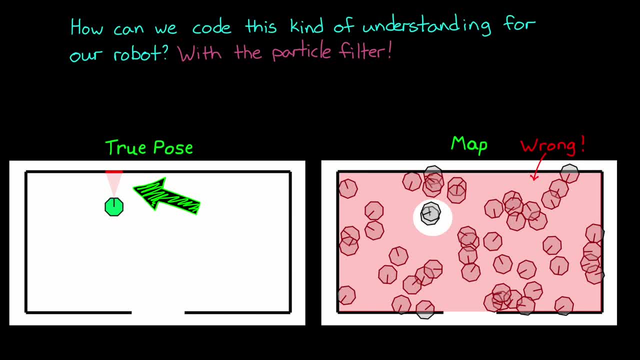 because at this point we're going to be able to calculate the probability distribution. At this point we get a LIDAR measurement and it returns, say, a pattern that looks like a wall. Now the filter can go through each of our particles, one by one. 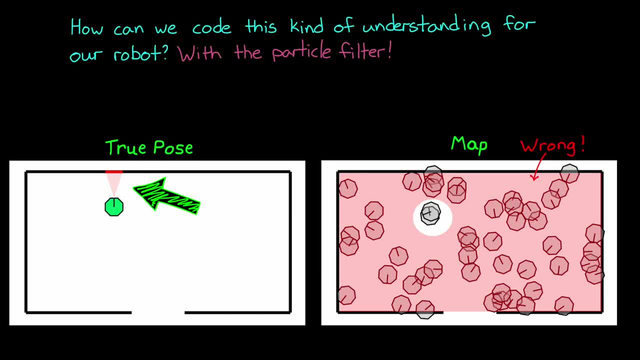 and determine, using the map, what the LIDAR sensor would have returned if that pose was the real one. Then it can compare the two scenes and determine how likely it is that the particle is the real system state. The closer the scenes match, the higher the probability. 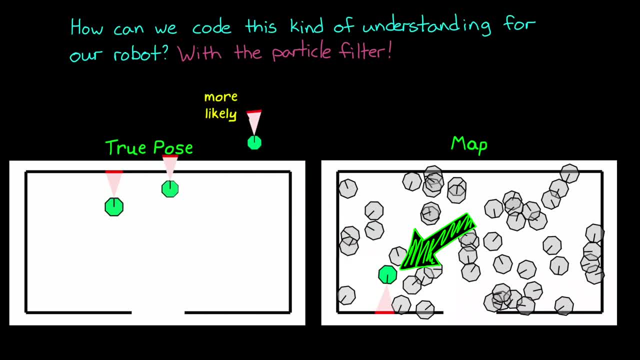 For example, this particle would return a scene that is much closer to what we saw than, say, this particle would. So I'm going to enlarge the particles that have a high probability of being correct so that we can see them better, and I'll shrink the particles that have a lower probability. 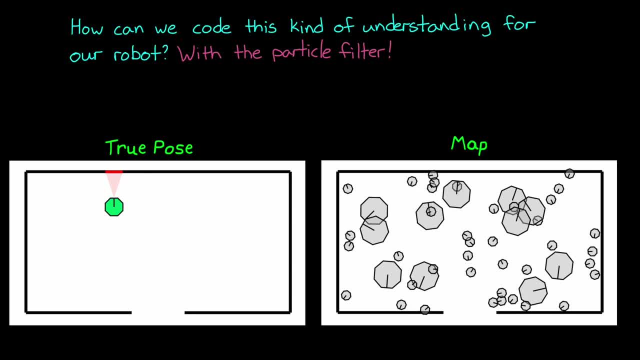 So, as we saw before, after just a single measurement our probability distribution is no longer uniform, but is skewed towards these more probable poses. Now we don't want to keep all of the low probability particles in the filter, since that would use up computational resources on unlikely poses. 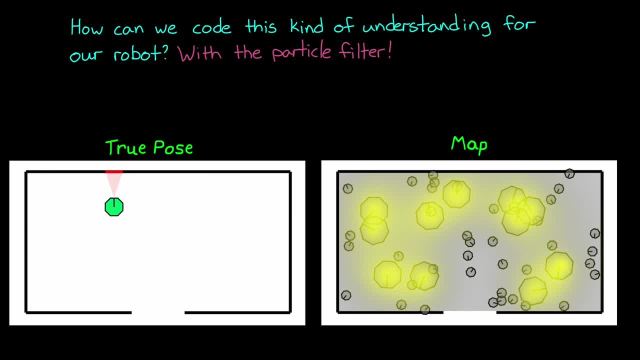 And we can also get into a situation where they cause the filter to never converge. Therefore, we're going to resample the particles according to this new probability distribution. This will place more particles in the poses that are more likely and less particles everywhere else. 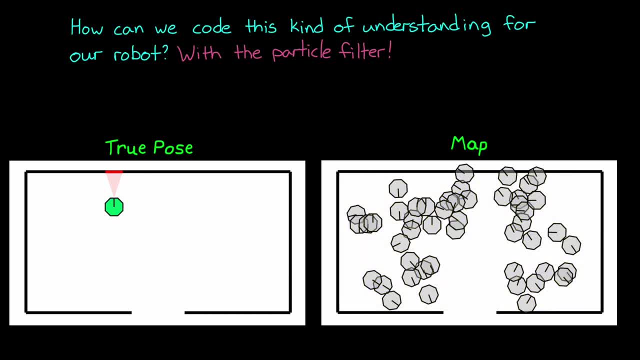 This random, discrete resampling of the probability distribution is why this type of localization is also referred to as Monte Carlo localization. Now, at this point, the robot is moving through the room, It's following the circular path that I showed earlier and it's dead reckoning its relative position through onboard odometry. 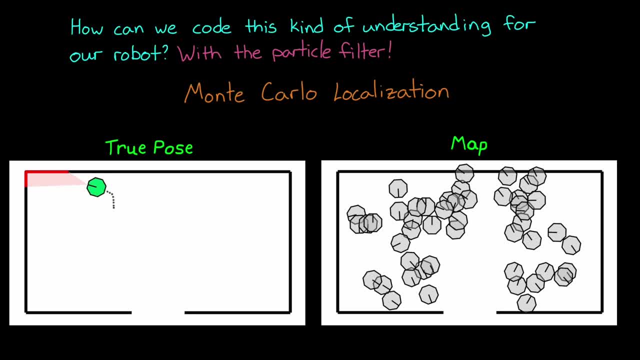 So the robot has a sense of how it's moving between LIDAR measurements and we can apply this estimated motion to every single particle in the filter. Basically, we're predicting where each of our possible poses go if they moved in the same relative way as the robot. 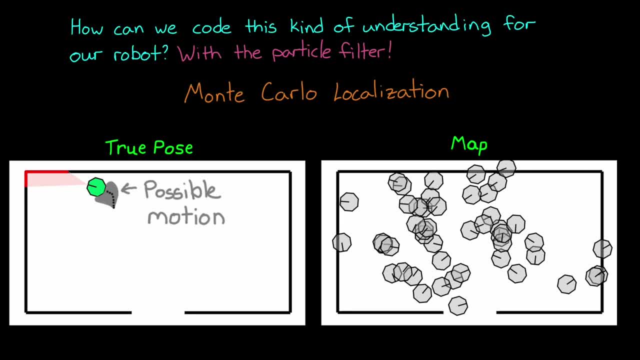 Of course I mentioned that dead reckoning is a noisy process, so we have some level of uncertainty in the estimated motion from the robot. Therefore, we don't just propagate each particle exactly with the estimated motion, but instead add additional random motion according to the process- noise- 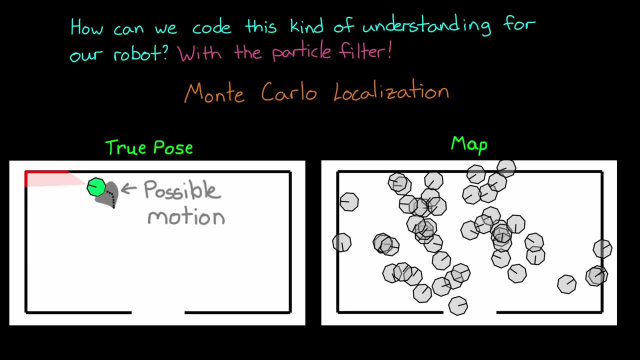 Some particles might move a little faster and some a little slower. Some turn more and others less. So here again, if the process noise is non-Gaussian, the particle filter can handle that. At least it can, At least as long as there are enough particles to accurately represent the distribution. 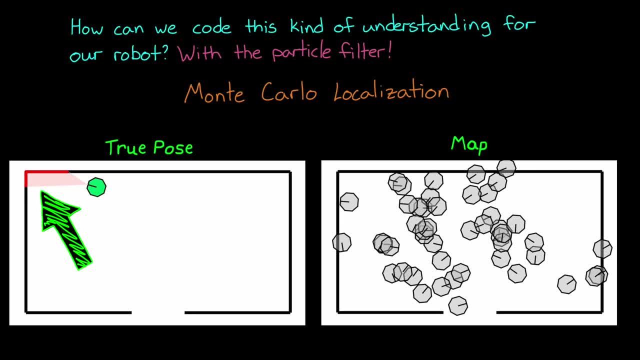 Now we can do the same step as before: We measure the scene with the LIDAR sensor and figure out which of these new particles are most likely to generate a similar measurement. The robot is looking at a corner now, which is good. 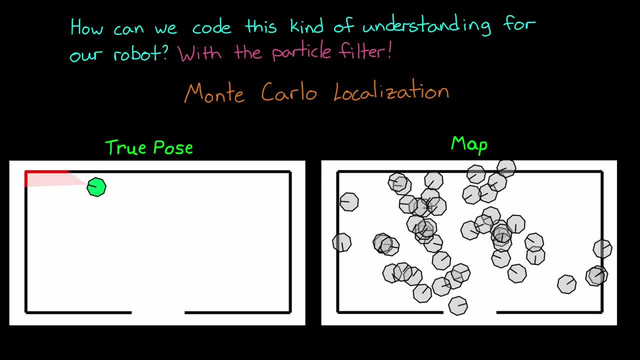 because that's a relatively unique feature in this map, But it still doesn't narrow it down completely. You can see that this particle is looking at a corner and this particle is looking at a different corner, So we can't tell just yet which is the real observed corner. 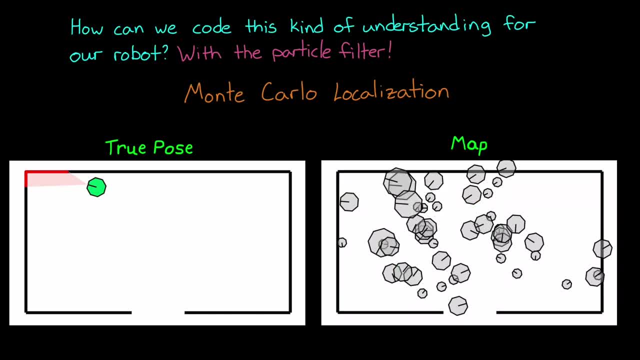 Once again, I'll enlarge the most probable particles and shrink the less probable particles, and we can get a sense of how the probability distribution has changed. Now it's bimodal, where there are two main possible locations where the robot could be. 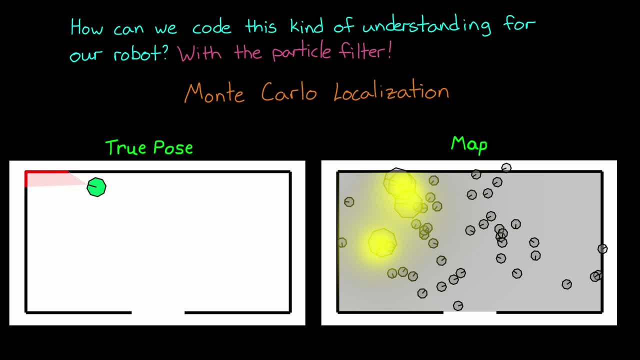 and everywhere else is a much lower probability. Once again, we can move on to the next generation of particles by generating a new batch of poses according to this probability distribution. But we can start to be a little smarter about it. For the first two generations, I used 50 particles. 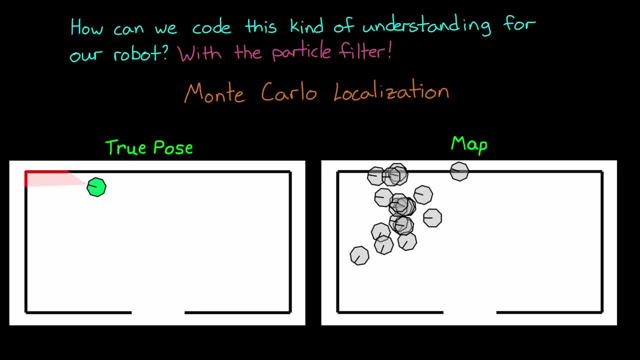 so that I could accurately represent the large and complex distributions. However, now that we're honing in on the real location of the robot and the distributions are getting narrower, it doesn't take as many particles to fully represent them. We could still use 50,. 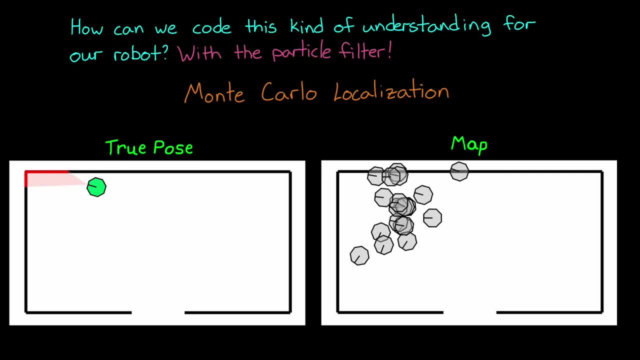 but that would just slow the filter down without adding too much value. Therefore, there is this idea of adaptive Monte Carlo localization, or AMCL, which recalculates the number of particles after each generation, so that you're not wasting computational resources. You do have to be careful about going too low with the number of particles. 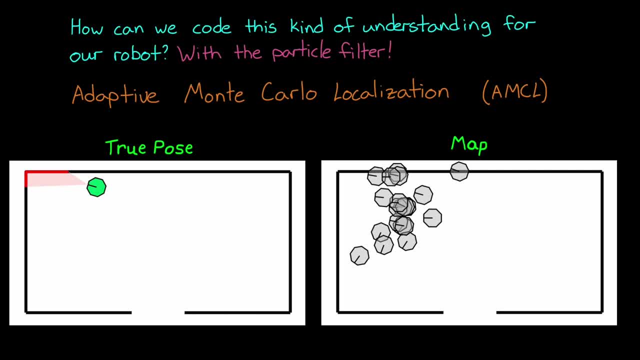 because the filter may get overconfident in its solution and misrepresent the true probability distribution, resulting in it converging on the wrong pose. So again, there's a trade-off here. Now the MATLAB TurtleBot example uses this adaptive Monte Carlo localization. 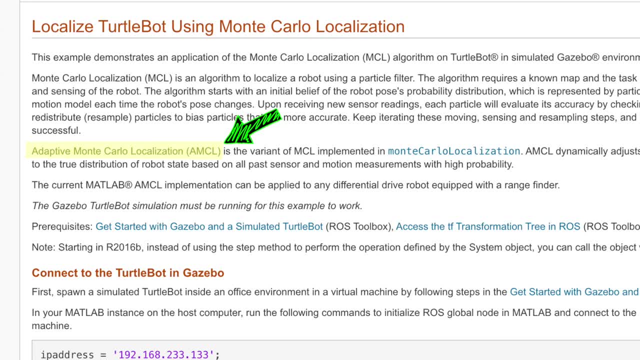 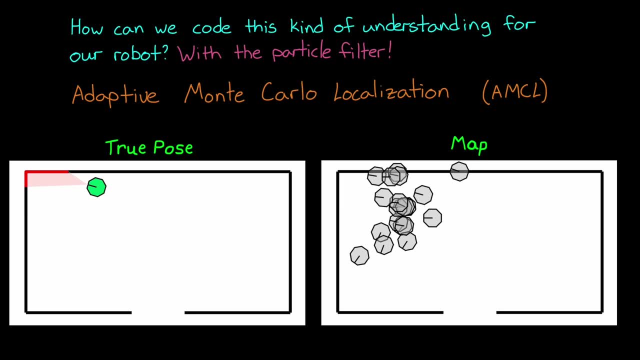 and there's a link below if you want to know the details of how this resizing is accomplished. Okay now, each generation is exactly the same as before. We model the motion of the robot using odometry. we apply that motion to the particles. 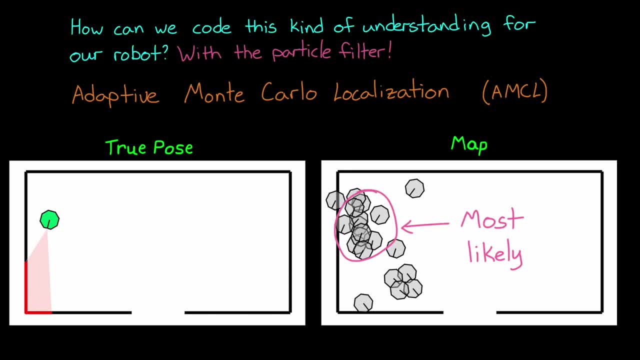 take another LIDAR measurement and determine which particles are most likely. Then we resample based on this new probability distribution and start again. And this iterative process is how we can use particles to converge over time on the actual pose of the robot. 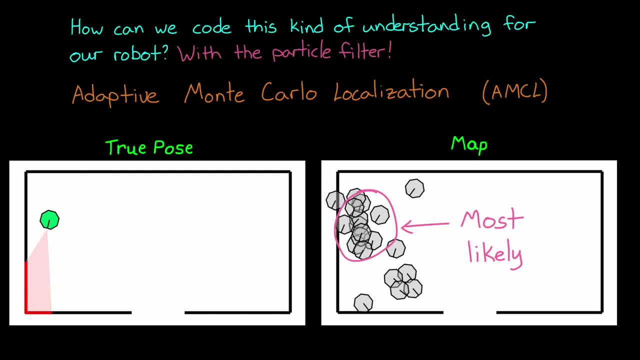 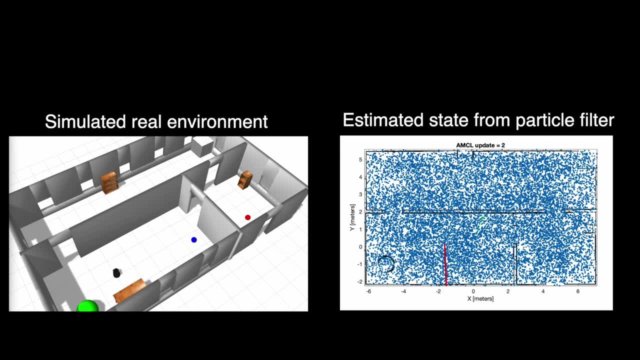 even in a room that is as featureless as this rectangle. So now, if we revisit the MATLAB example from the beginning of the video, it should make a lot more sense as to why these blue dots are here- They are the particles- and why they're moving around each iteration. 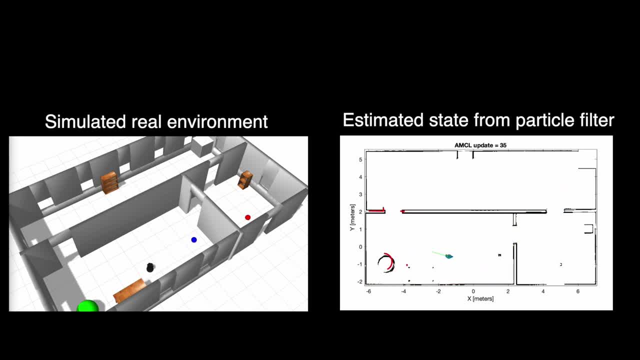 and why the number of particles is getting smaller as it converges over time. This is the particle filter at work in the adaptive Monte Carlo localization approach. Now, I think, a good way to get a better feel for how all of this works and how you can implement it in MATLAB. 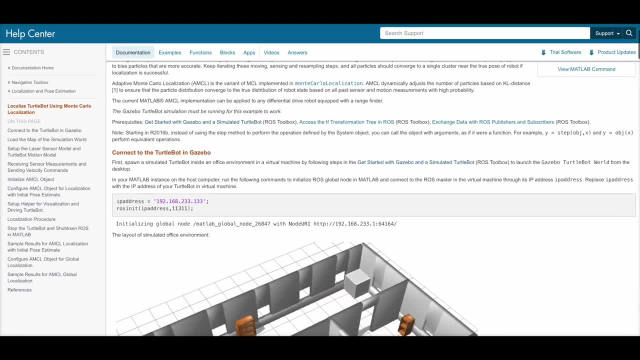 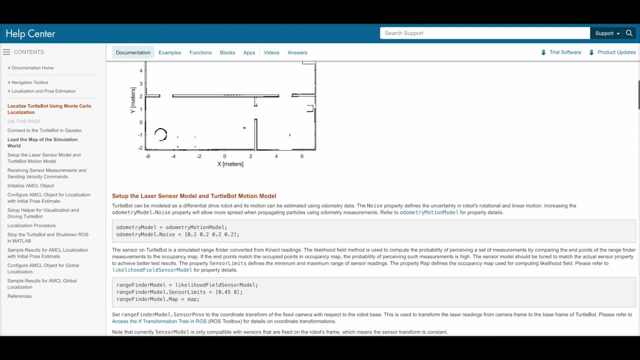 is to just play around with this example. You can change some of the filter parameters and see how it impacts the solution, And you can check out the different functions that implement each of the ideas that we just talked about. Then, when you go to learn the mathematics behind it, 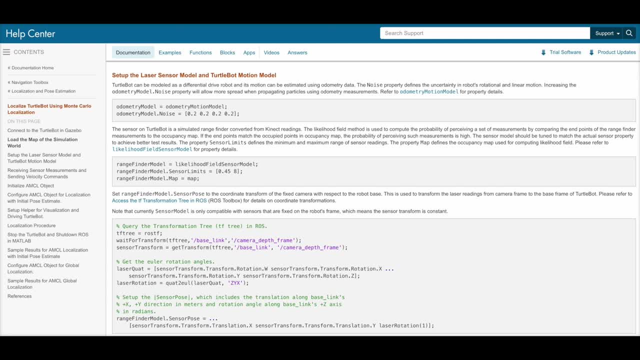 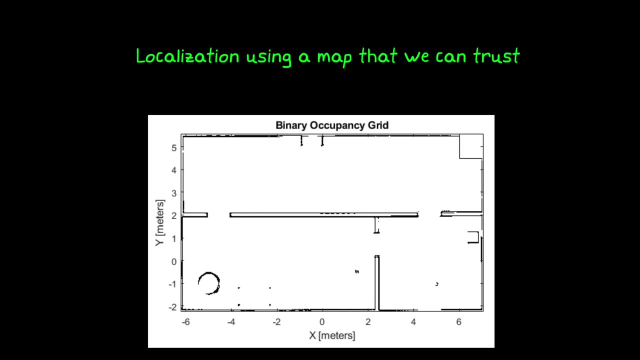 you'll already have this intuitive feel for how the filter works and hopefully the math becomes easier. Alright, in this video we really only looked at localization, assuming we already had a map that we could trust. But what if that's not the case?